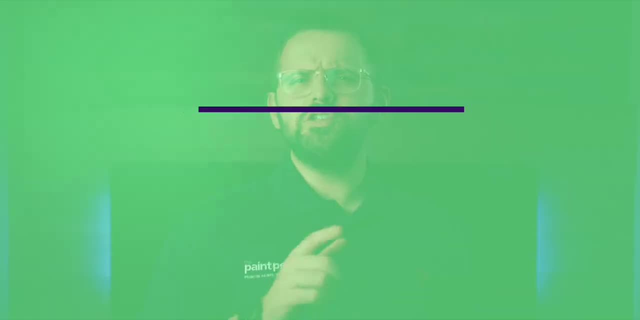 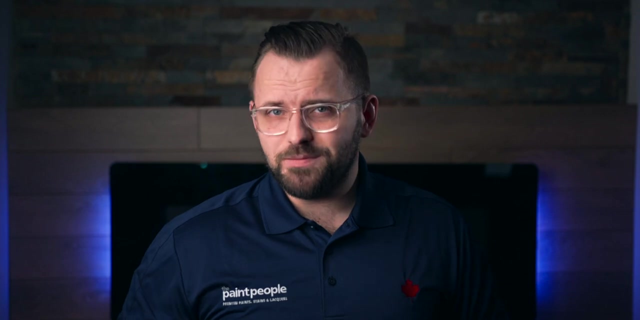 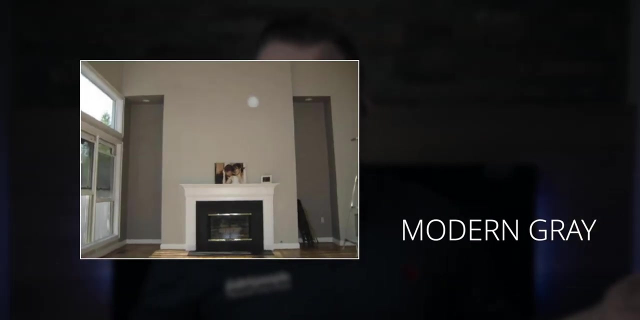 the French word for mole. Fun fact, Where should you use it? If you're wondering whether or not this color is too dark to use throughout your entire home, I don't blame you, because it really is a tough call to designate this as a main color candidate. It's certainly user-friendly and has that wonderful balance of. 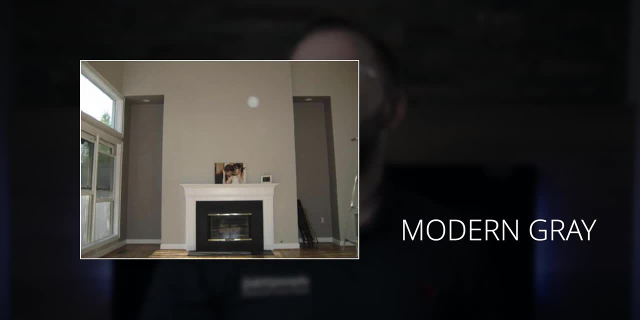 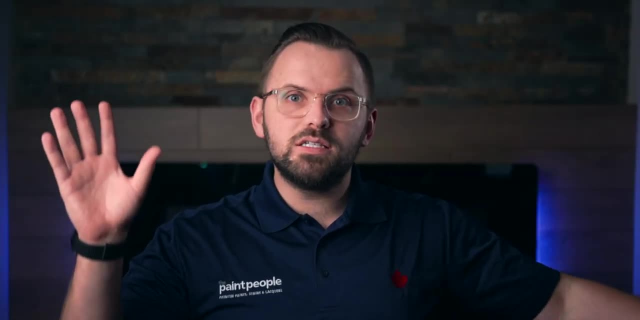 inviting beige warmth, but it's definitely on the darker side, especially if you use it in those poorly lit areas. This isn't going to be the color choice for someone looking for a minimalist look, but if you were thinking of using a white or an off-white anyway, you probably wouldn't have 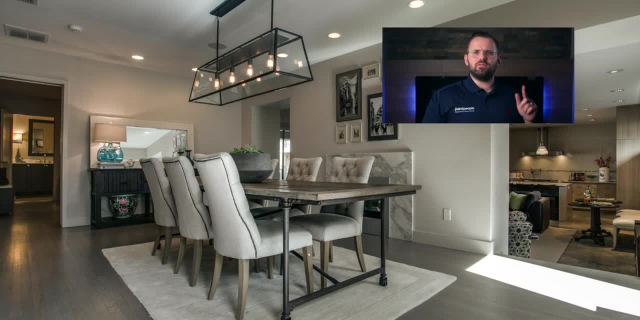 clicked on this video. Modern gray is an ideal choice in areas that have a lot of light, have a lot of white woodwork or surrounding fixtures to counterbalance it, or those areas where you want a little bit of drama without shoving it in people's faces. It's all about perspective, after. 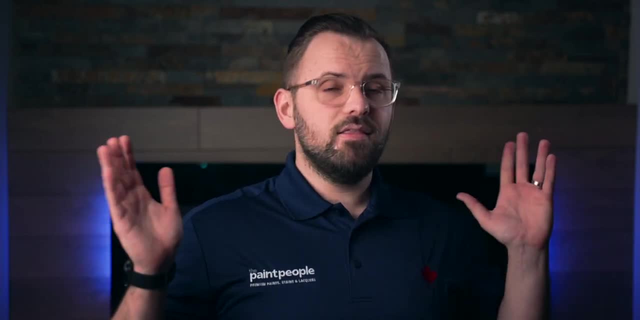 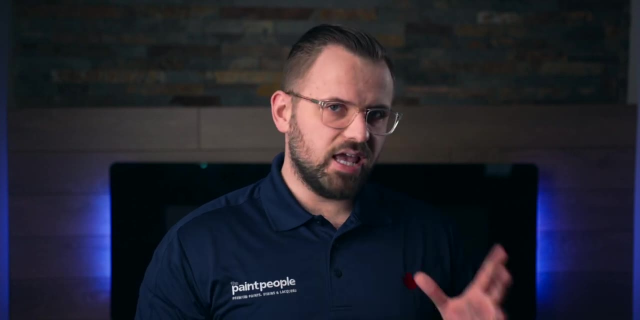 all. If you're used to using white all over your house, then yeah, modern gray will feel a bit dark. but if you've been comfortable using darker taupes like dovetail or some more bold browns or charcoals, then modern gray will slot in nicely. 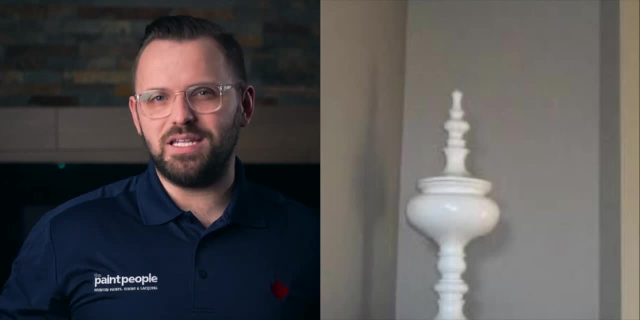 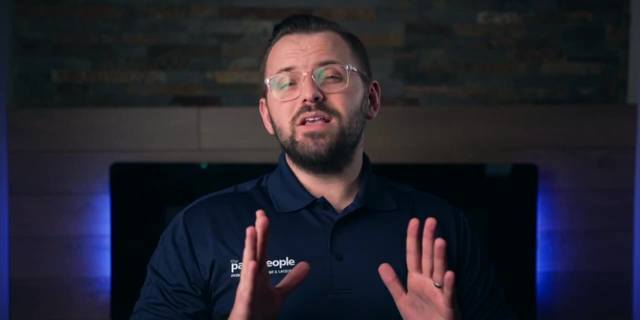 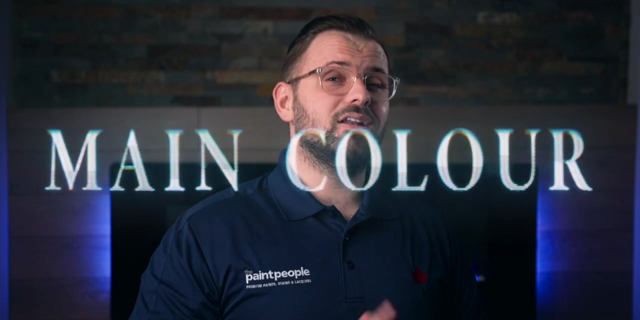 as a lighter, neutral canvas color. The one thing that can't be denied is that LRV we talked about earlier. It's going to be darker than any off-white out there. Just based on its undertones alone, this one just barely gets my main color stamp of approval, but I award that distinction with. 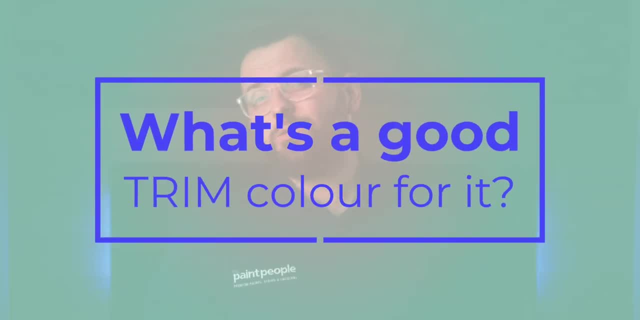 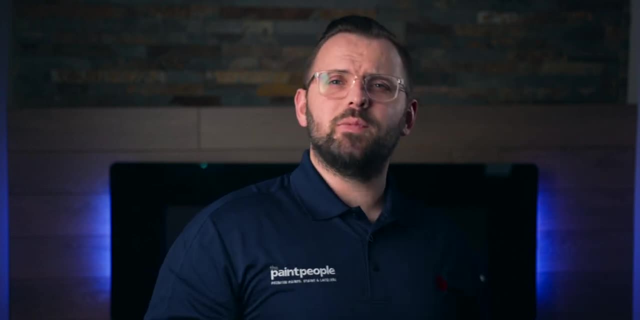 an asterisk, What's a good trim color for it? I don't need to rely on my own creativity too much here, because Sherwin-Williams has already given you an answer. Looking at the Sanctuary color palette, that modern gray was taken from. 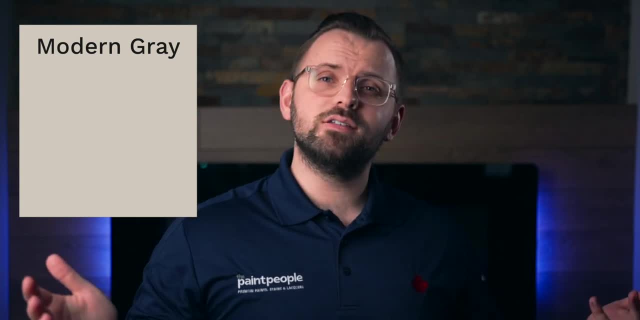 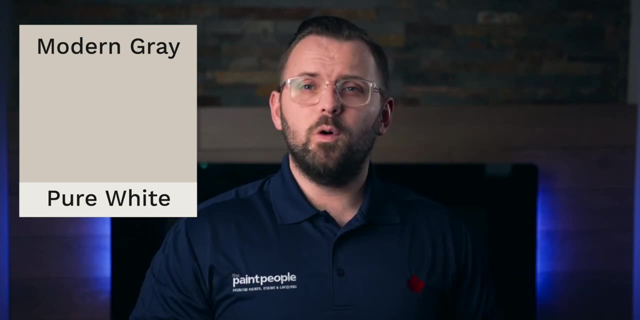 you'll also notice a white in that grouping as well, and it's called pure white. Pure white is great because it coordinates really nicely with any of the neutral color palette, whether that would be on the cooler or on the warmer side of things. Ironically, it's not exactly a pure white. 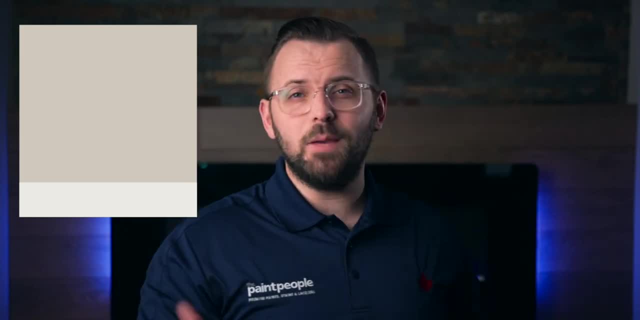 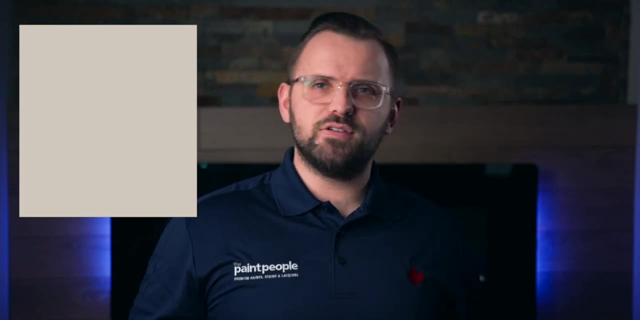 but its impurities, with its dash of gray and cream, allow it to fit itself perfectly into modern gray, like a jigsaw piece. They're just made for each other. You could also opt for something a little more airy, like an off-white called white snow. This. 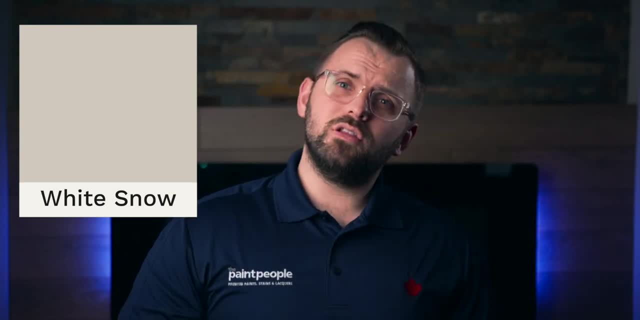 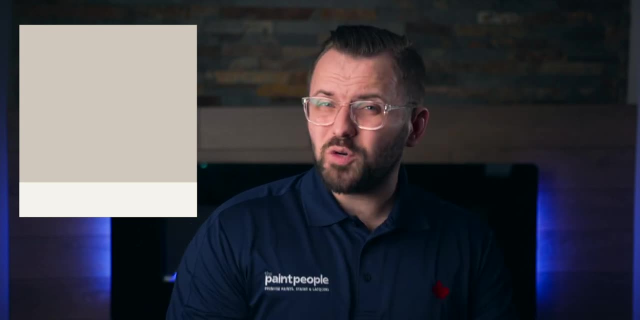 one will feel quite a bit brighter. It'll pop a bit more, which could look quite nice on your more low-profile woodwork and trim. but if you're painting more large-scale wainscoting that you want to feature prominently, I would probably opt for pure white, because it will be more of 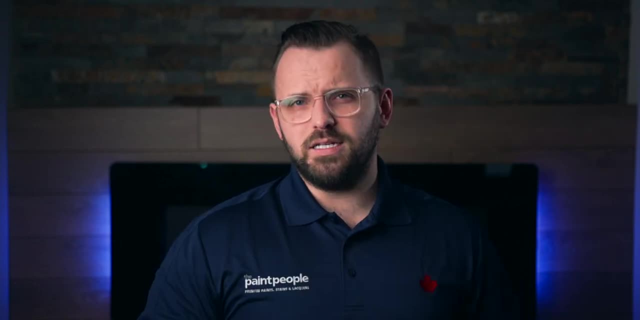 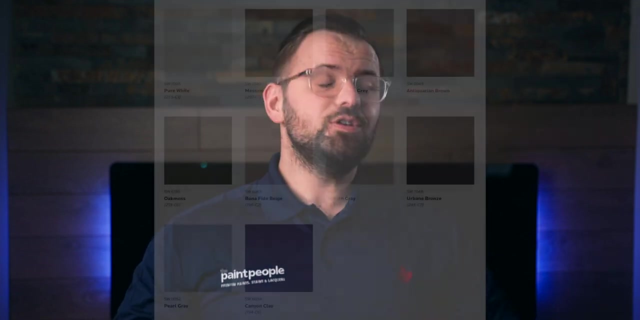 an inconspicuous look which, to me, feels a little more refined. What are some interesting color pairings for it, Other than steering you towards the previously mentioned sanctuary color palette, which would be a wise move, considering they were all hand-picked to go together? 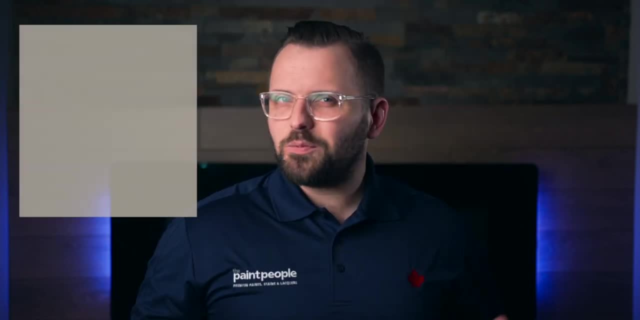 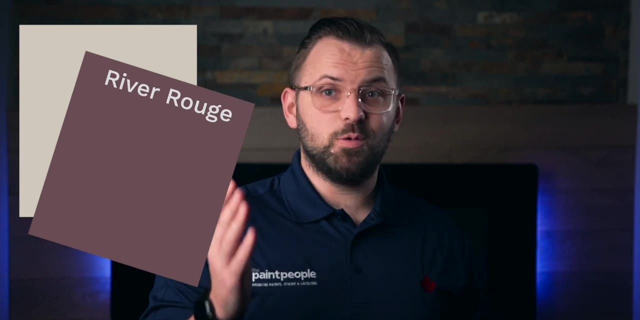 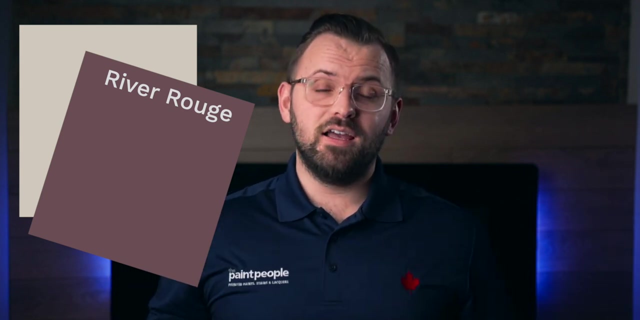 I would present another option to you and it's sort of a fun approach to taupe. Take a look at River Rouge, which is, for all intents and purposes, a dark color. It has a 12 LRV, but I love it because it satisfies that dark, neutral accent color. that is anything but boring. I just love. 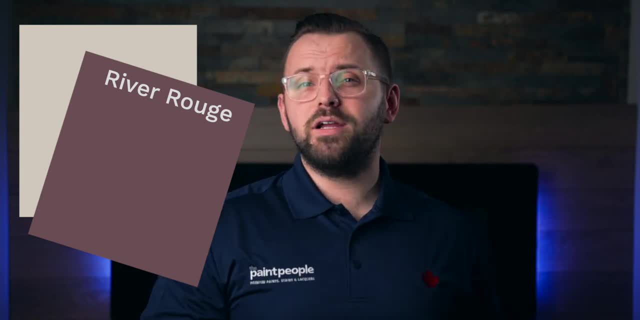 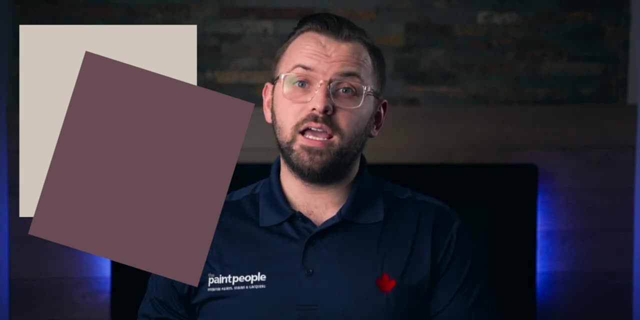 its plum burgundy undertones. I think it's a great color to go with any color palette. It's a really fun complimentary color that seems to add the right amount of color and also does a good job at working alongside the bit of red found in modern gray. It would be a dramatic choice for. 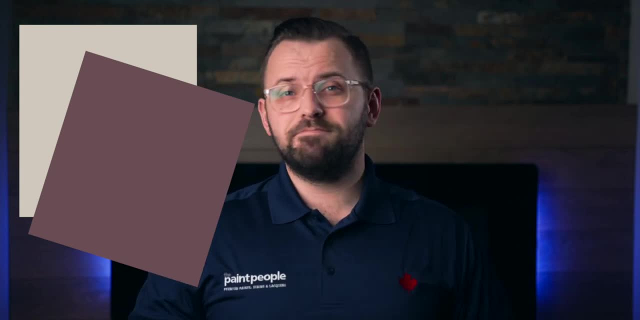 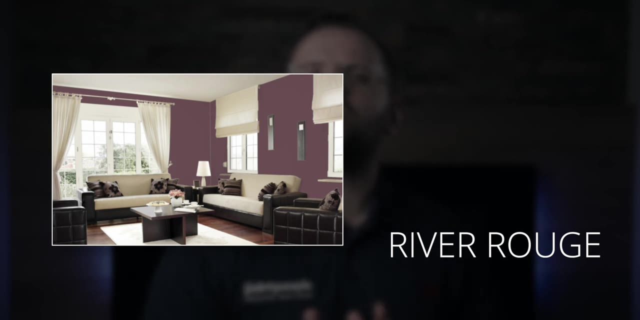 an entire room but would suit a powder room perfectly, and even in larger rooms, because to me anything that is on the warmer side of things will always feel a little more cozy and welcoming compared to a colder color alternative. Can you compare it to other colors? Of course I can. It's not like there's a lot of detail in every color, but I like them. I think they're both fairly well-made colors and I like how they're all matched. They're both the same color, but in some ways they're the same color but not the exact same color, So I'd like to see that they match each other. If you're just putting a lot more evidence here, then of course you should make a few corrections to that, of course. 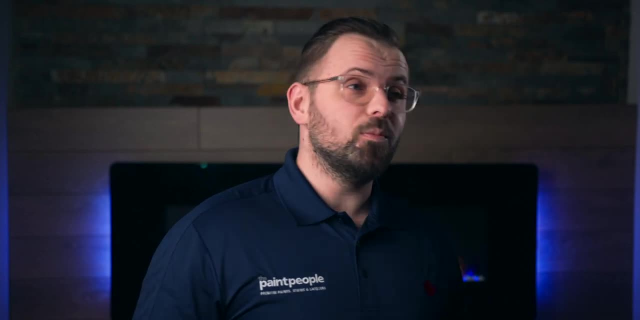 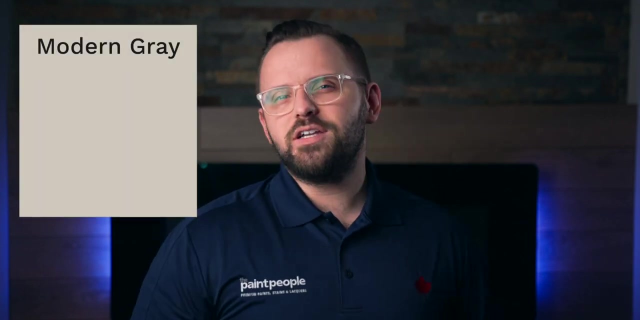 Of course I can. It's not like there's a shortage of mid-tone, warm neutrals out there, am I right? If you were looking for something that was a little bit warmer and had even more of that beige, then I have a color for you that has one of the best names I've heard in a long time. 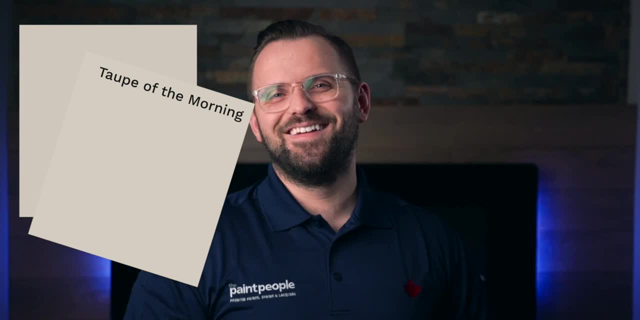 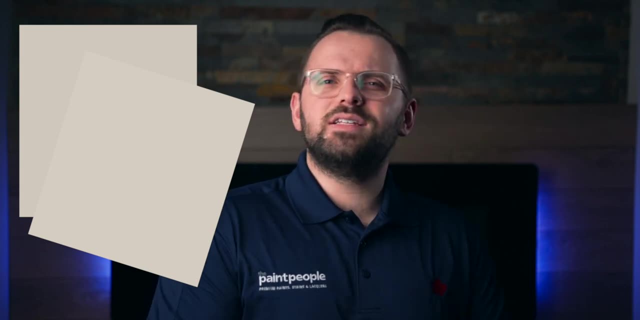 Taupe of the Morning. How amazing is that Similar color here? It's a touch lighter than modern gray and will feel even lighter because of its added gold hue. If you wanted to take a few steps in the other direction and go a little more towards brown and taupe.